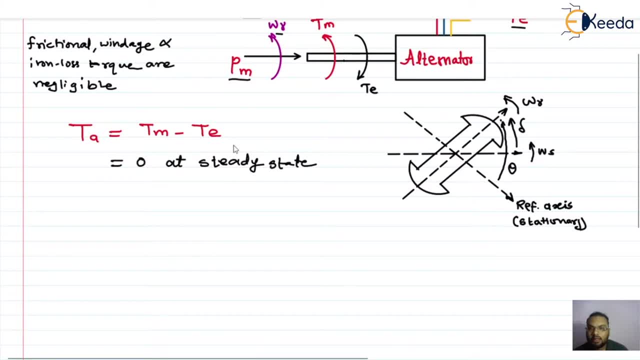 equation as equation number one. if I multiply this equation over one with the respect to this angular velocity, that is Omega r. so I will get here as Ta mod. omega r is equal to Tm x. omega r minus Te into omega r and we know that for torque into 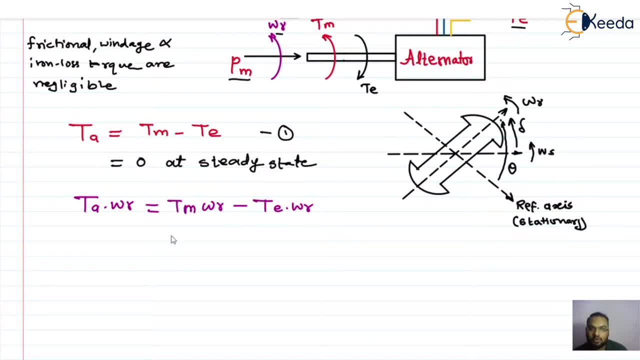 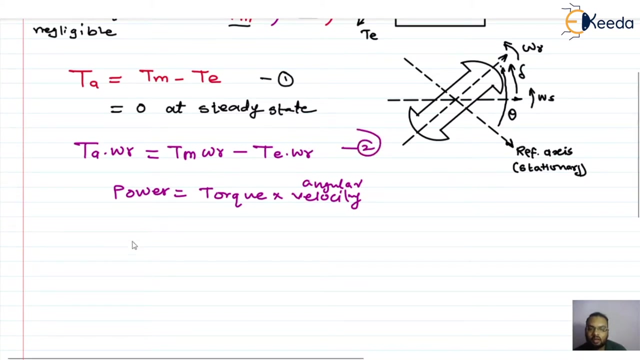 velocity will give us the power. so as for this, I can write here, as power is nothing but torque into, definitely it will be an angular velocity. ok, so from this we can write. as for this equation, number 2 I will get here, as Pa is equal to: 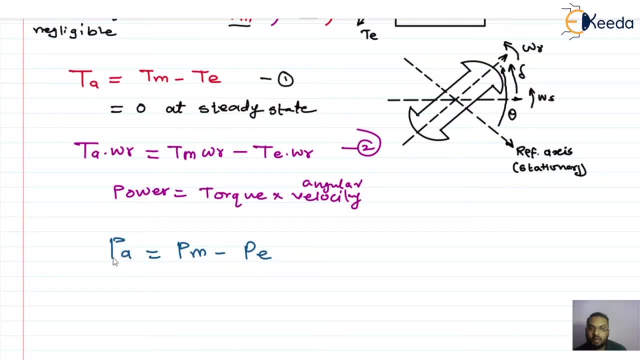 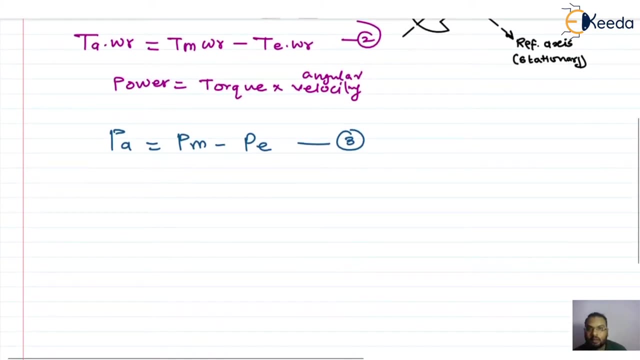 Pm minus Pe, this Pa is the accelerating power, Pm is the mechanical power and Pe is the electrical power. ok, let me write this as equation number 3. ok, now, this Pa, it is the accelerating power. ok, and we can write it as: Ta into omega r. 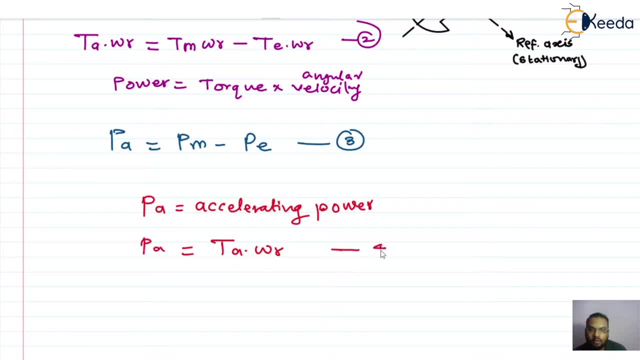 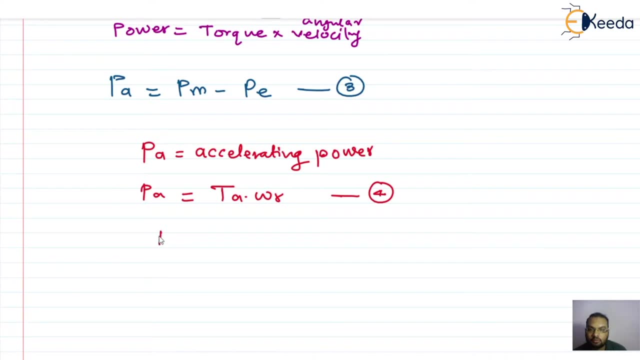 Ta into omega r. ok, now this Ta, I can write it as J into alpha. how this J- we know it is a moment of inertia- into alpha. here this alpha is angular acceleration, ok, and of course this J is moment of inertia, ok. so as for this, I can write this: 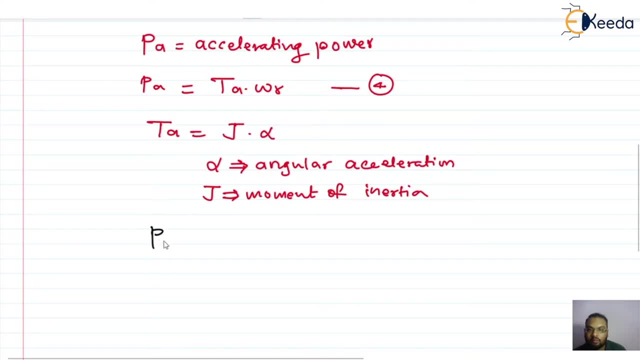 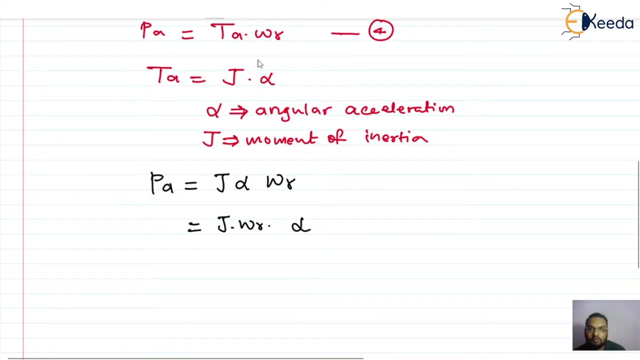 Pa, that is, accelerating power. as Pa, it can be written as J alpha omega r. let me rewrite it as J omega r into alpha ok, why? because because we know that this J into omega r, it is nothing but m. ok, if you remember this from the previous discussion. 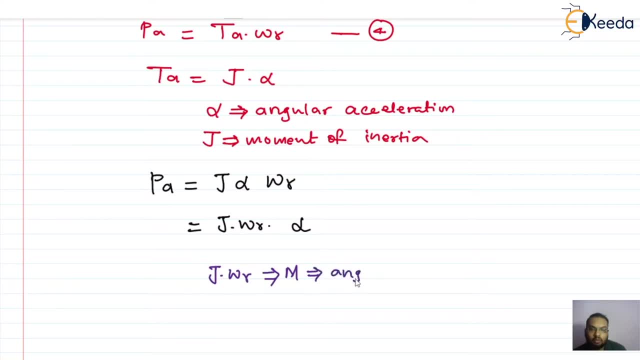 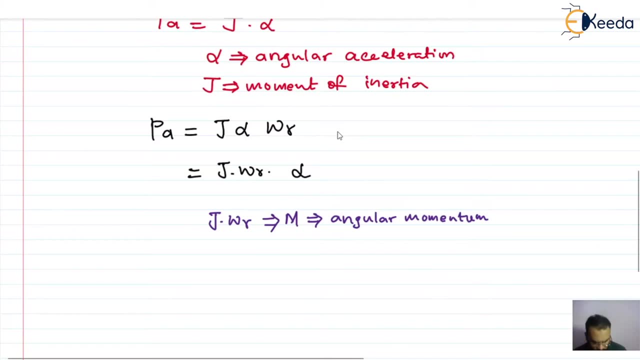 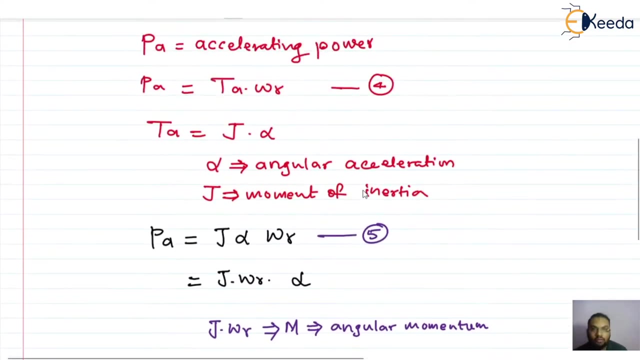 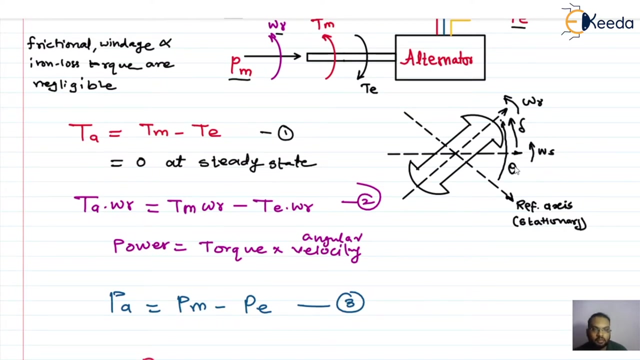 that m is nothing but angular momentum. ok now, taste of É. now, let us call this as equation number five. ok now let us get back to this diagram. here, this Theta is nothing but the angular displacement. ok, now I want to write this in terms of this synchronous angular 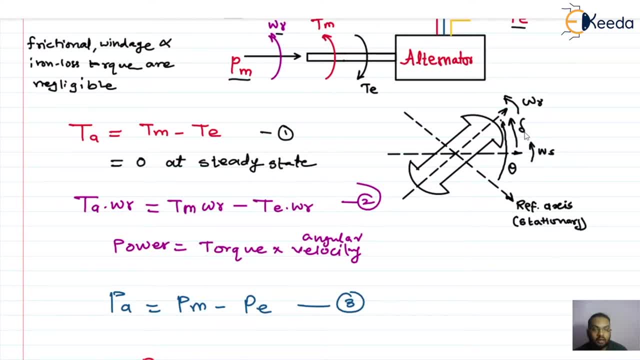 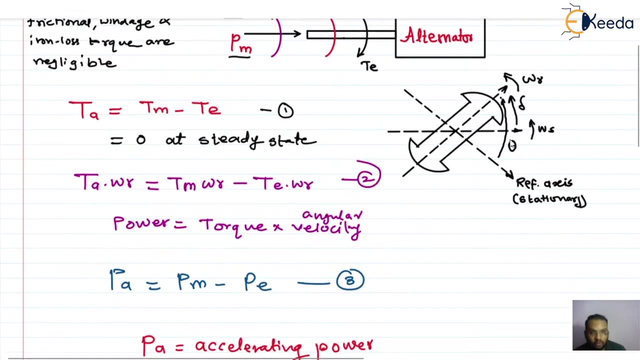 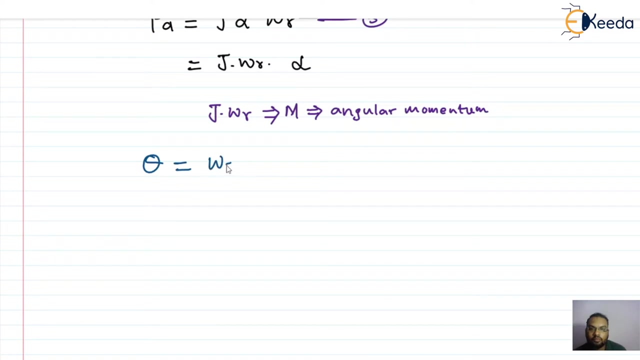 speed and this rotor angle, Delta. ok, this Theta, it is now from delta, this theta it is simply, it is a combination of this position of this axis at time t plus this delta. okay, so, specifically, in terms of mathematical form, i can write this delta as: omega s t: position of this axis which is rotating at synchronous speed at time t. 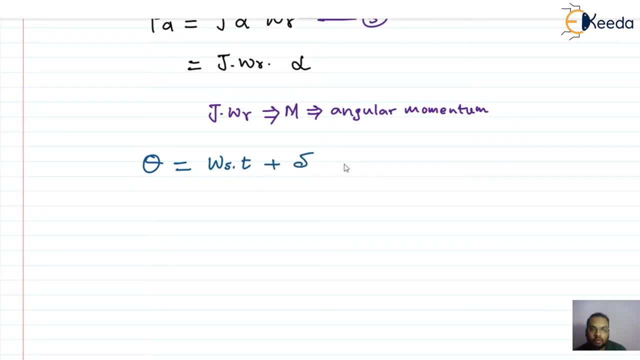 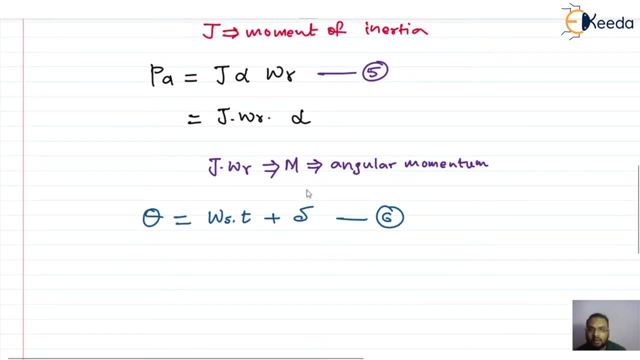 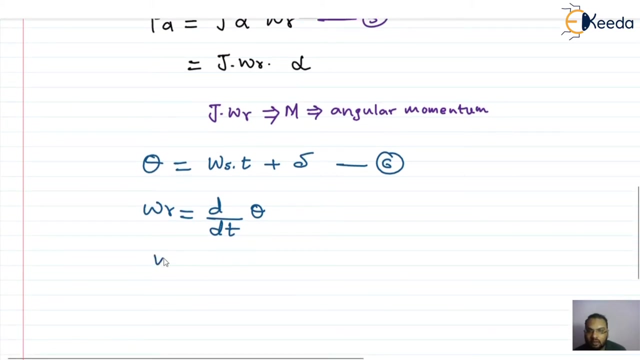 plus this delta. okay, all this as equation number six now, from this angular displacement. how do i get this angular velocity? angular velocity is simply d by dt of this angular displacement. so, as for this, can i write omega r as d by dt, by dt of omega s into t plus this delta. okay, if i open this bracket, if i differentiate these terms, 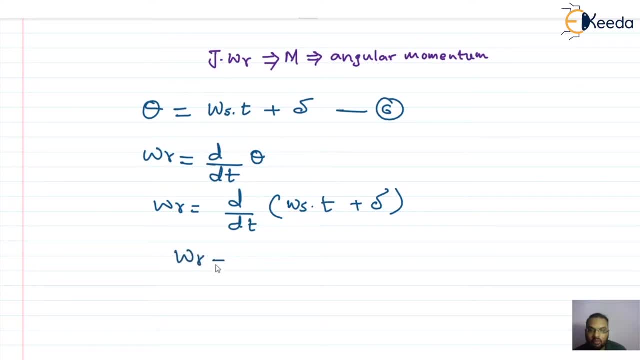 so this uh, i will get here as angular velocity of the rotor. it will be, see this, d by dt of this term, this time, d by d uh, d by dt of this time will be one. so omega s, it is a constant, okay. plus, we will get here d by dt of this delta. okay, let me call this as equation number seven. now here. 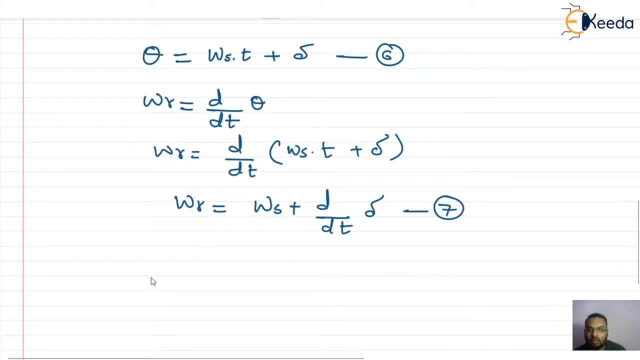 now from this angular velocity. now i want angular acceleration, so that angular acceleration alpha. we will get it with the help of this one d by dt of this omega r, okay, but no doubt this omega r is actually d by dt of this t. so we, i can say here, as this angular acceleration is nothing but. 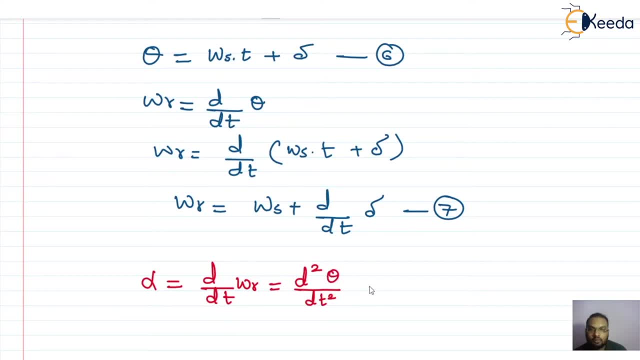 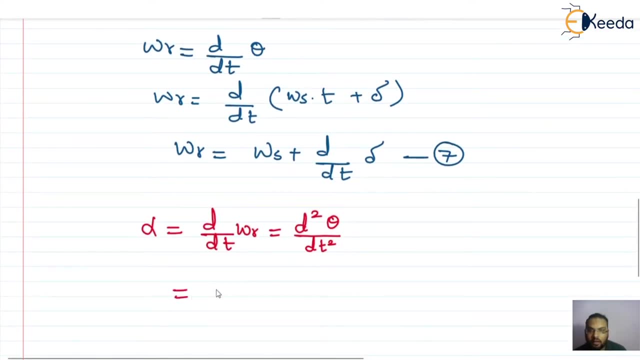 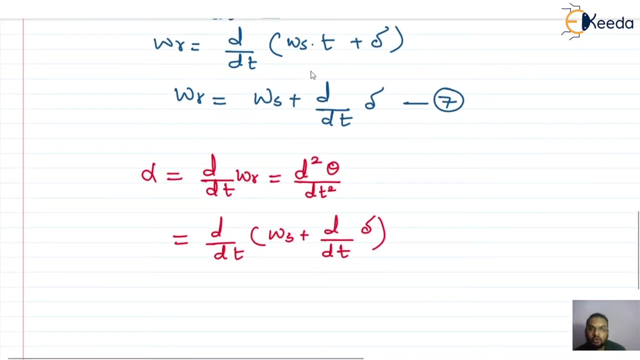 d2 by dt square of this theta. okay now, furthermore, let us solve for this: d by dt of this omega r, d by dt of omega r is nothing but omega s, plus d by dt of this omega r, d by dt of delta. okay, so from this, this omega s is a constant, so we'll get zero here, plus d by dt of 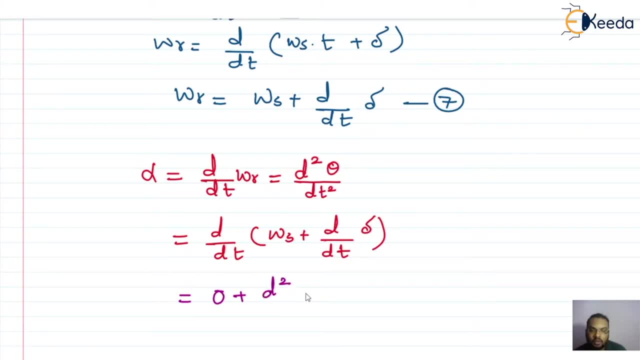 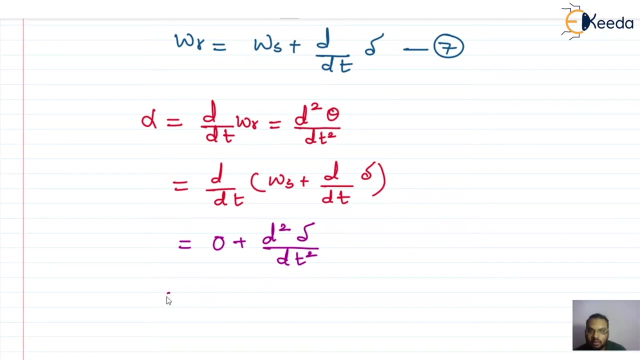 d by dt of delta. so we will get here d2 delta by dt square. okay, so if you compare these two equation, this alpha and this equation, so i can write it here as alpha is nothing but it is equal to d2. theta by dt square is equal to d2 delta divided by. 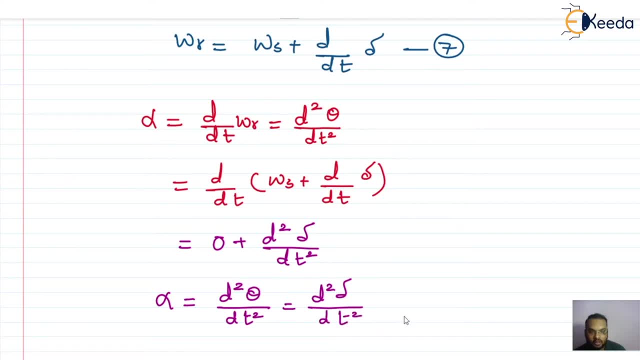 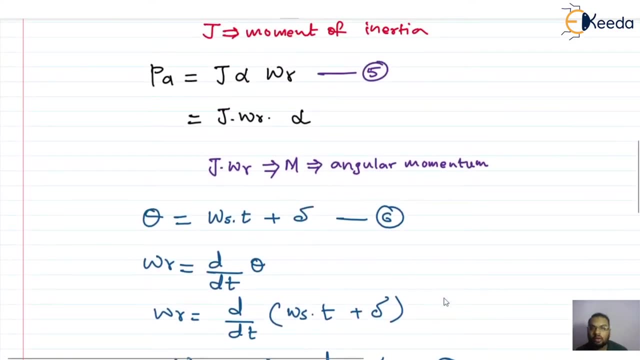 dt square. okay, let me call this as equation number eight. okay, now you get. look at this equation number five. okay, so in this equation number five, instead of this alpha, i'll write that term. okay, so here we will get this equation number five. okay, so in this equation number five, 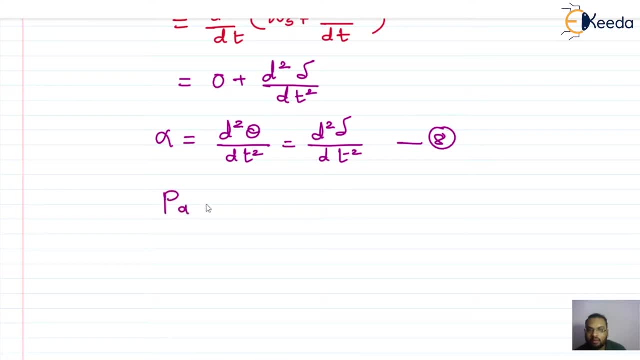 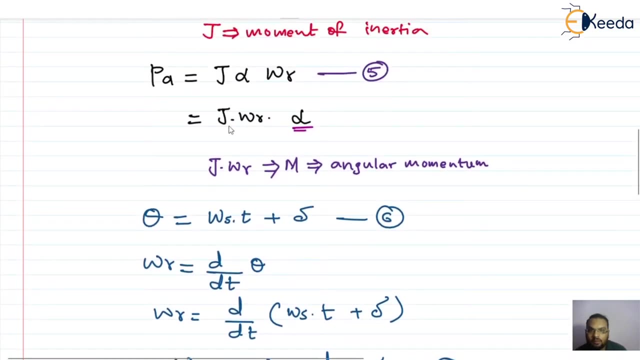 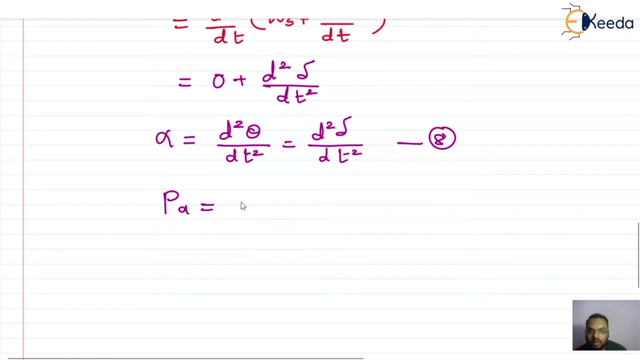 we will get that power. accelerating power is equal to again if i replace this j into omega r with m. so i will get here as. let me write here first: as it is j into omega r, into alpha, so it is, as per equation, number five. So this j into omega r is nothing but m and this alpha I can write it as d2 delta by dT square. 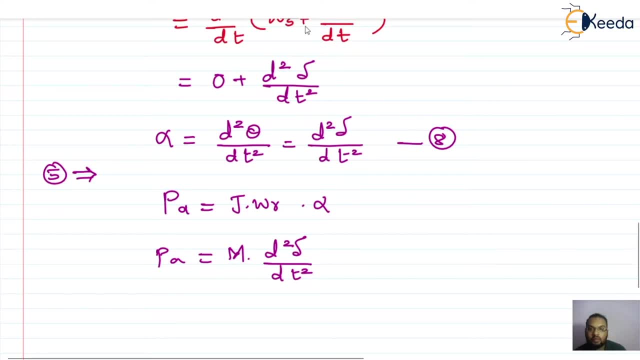 Okay, this is P A and this equation is nothing, but it is called as the swing equation, Okay, and furthermore, we know that this P? A is nothing but P m minus P e. Okay, so this equation is the swing equation of the synchronous machine. 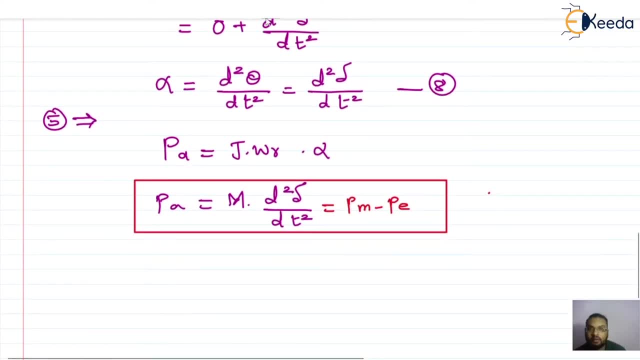 Okay, how we can define this, How we can define this swing equation. You can easily see that it is a second order differential equation. Second order differential equation. Okay, what this differential equation is giving It is giving us. it describes the relative position of this, or the relative motion of this delta with respect to the rotating axis, which is a function of time. t. 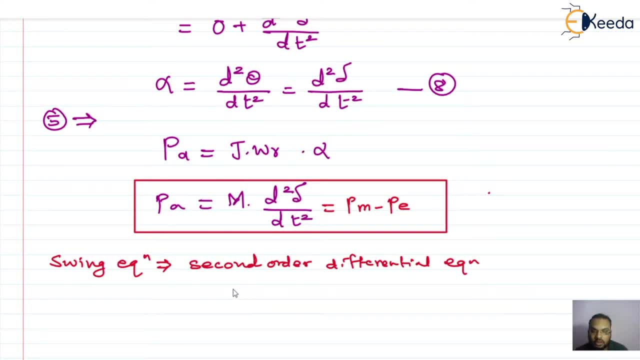 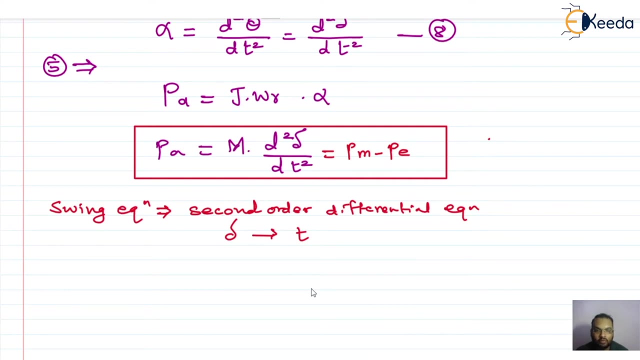 Okay, simply, we can say that it is giving us the relationship between this angle delta and the time t. Okay, from this swing equation We can plot the swing curve for the synchronous machine. Okay, before going to the swing curve, Let me add one more point here. 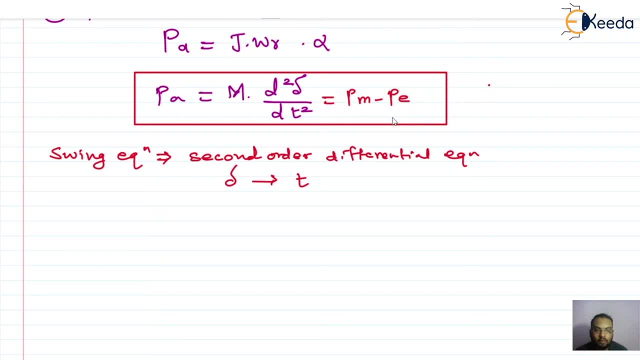 In this swing equation. In the beginning we have neglected some torque. Those were frictional torque, windage torque, iron loss torque. Okay, again, we have neglected the damper winding as well here, If suppose, if I want to include that damper winding as well here. 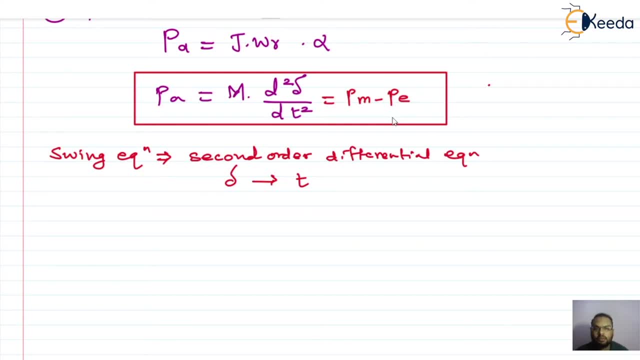 So I can add the damper winding in the in my stability studies, which is because we know that the damper windings they provide the better stability for the synchronous machine. So sometimes it is given or it is asked to include that damping power in this swing equation. 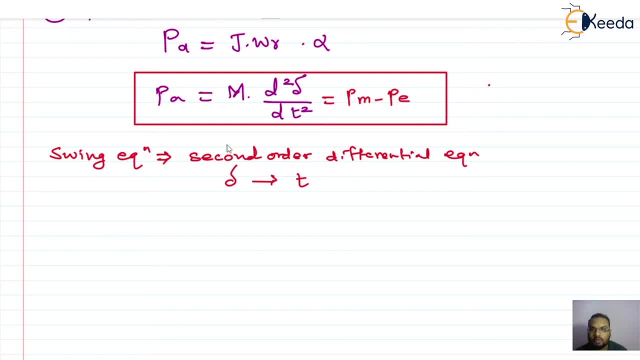 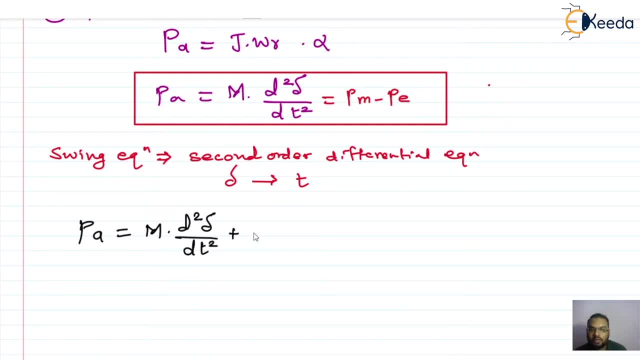 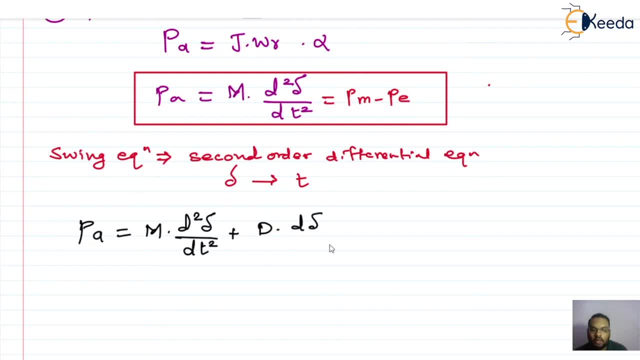 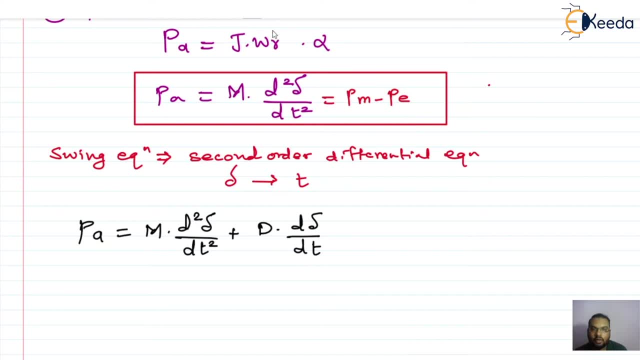 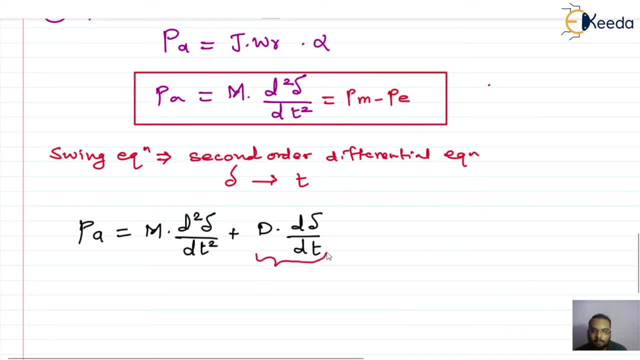 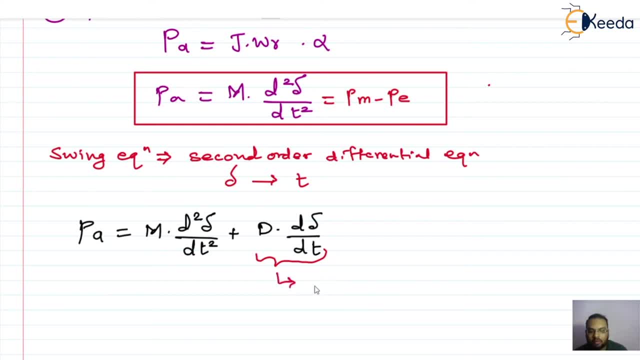 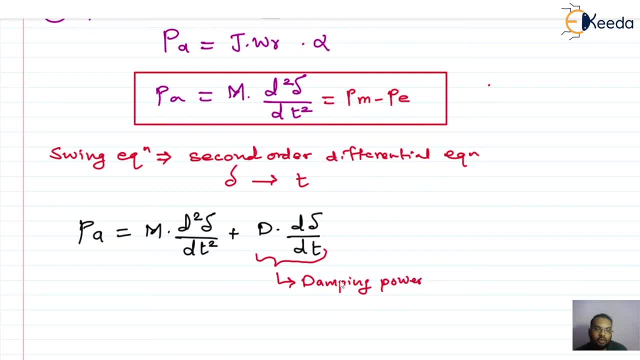 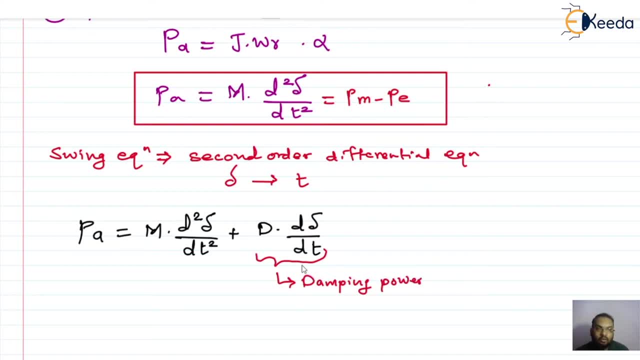 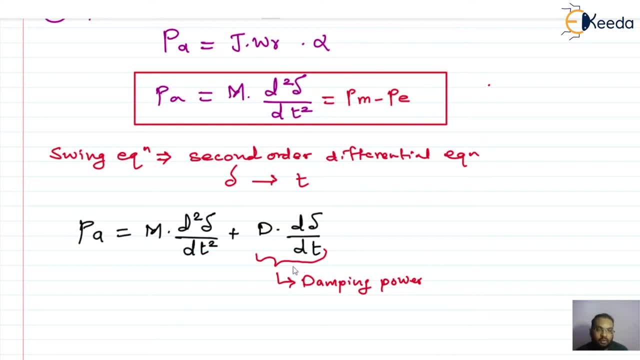 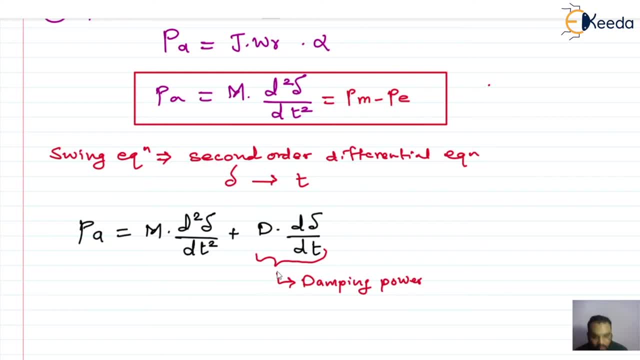 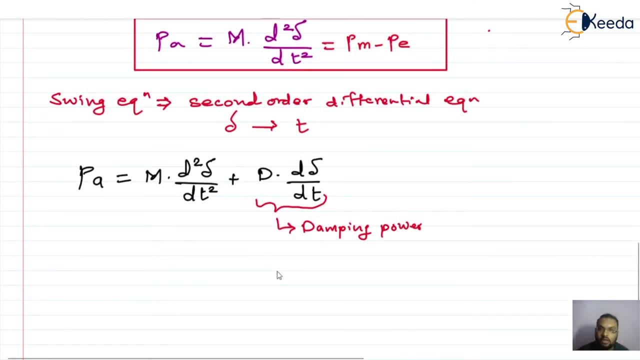 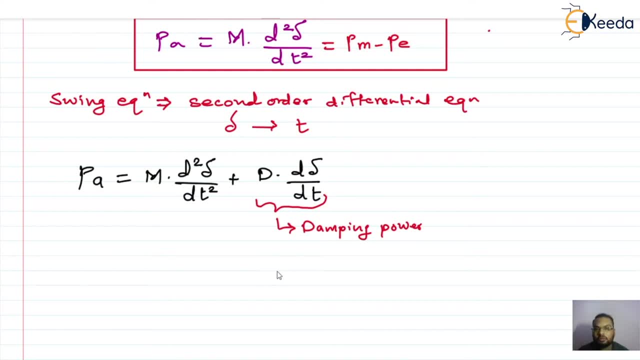 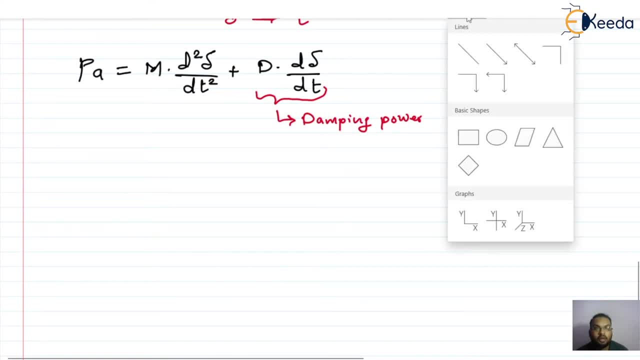 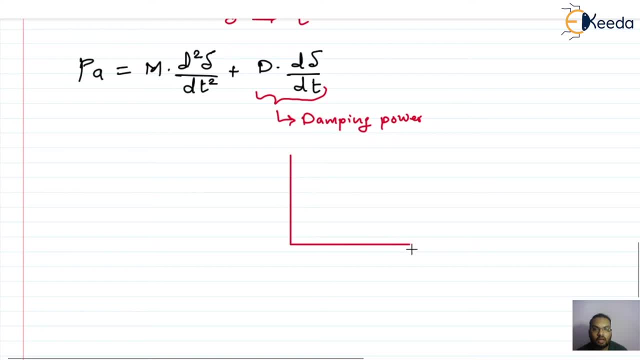 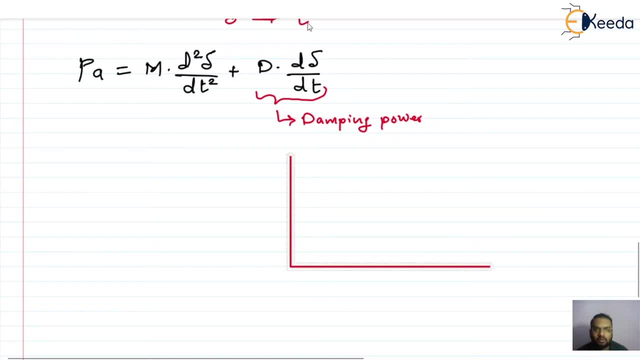 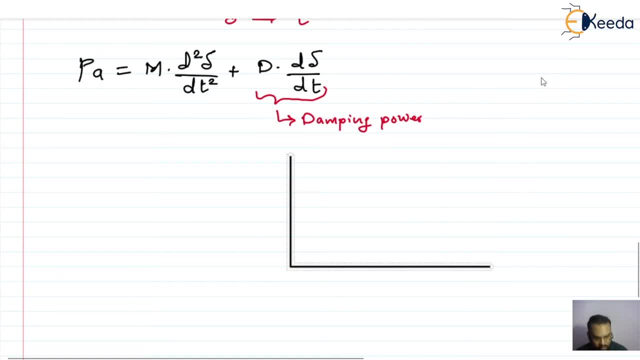 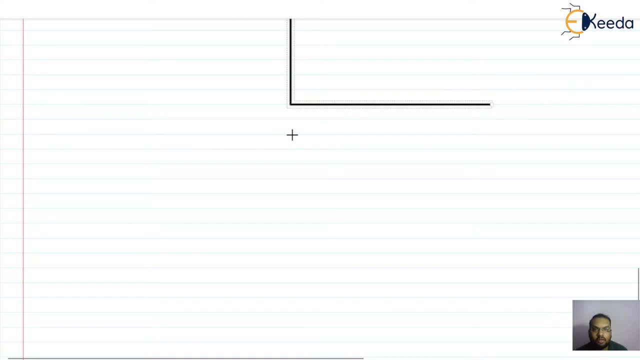 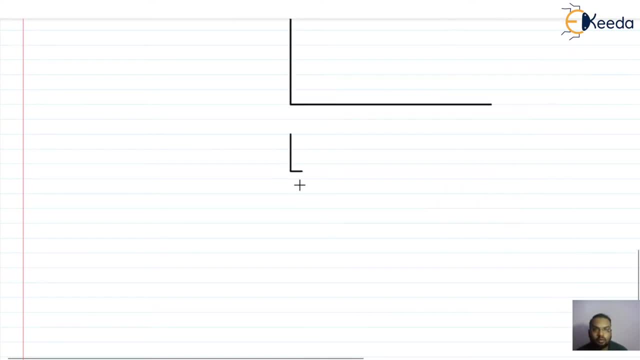 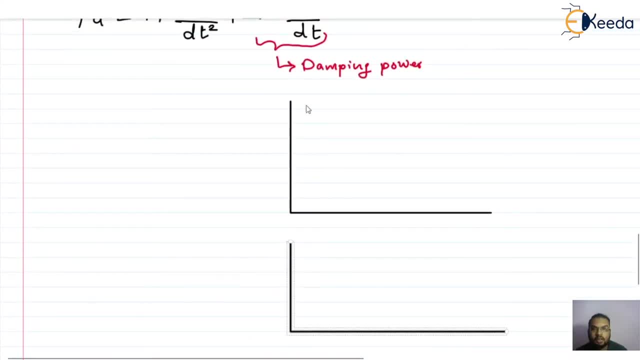 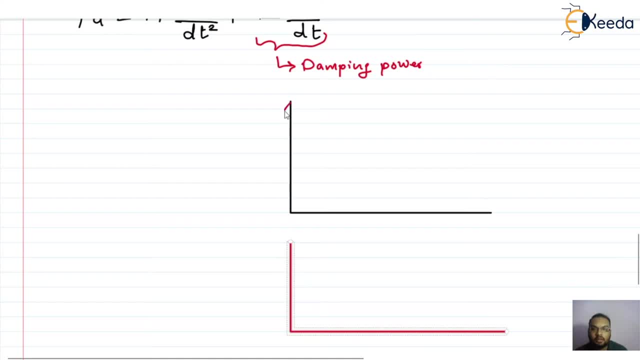 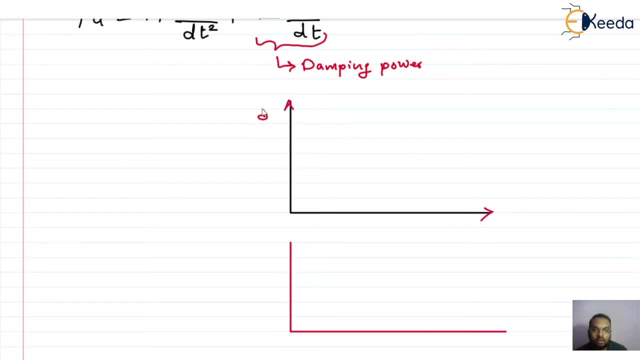 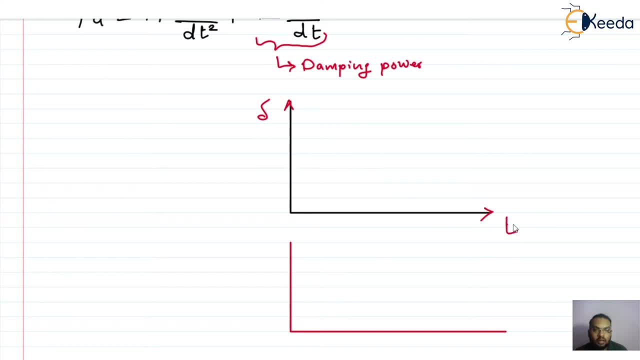 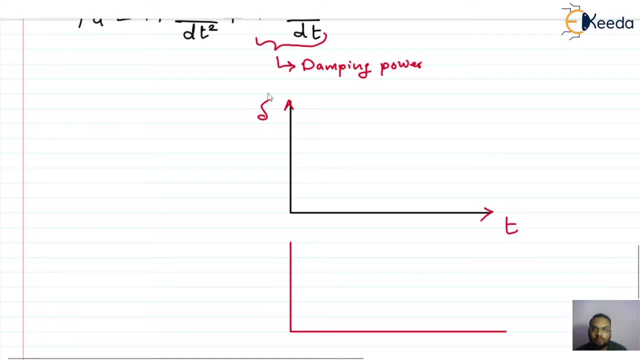 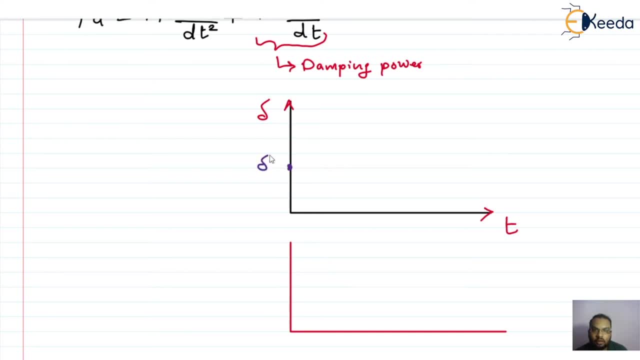 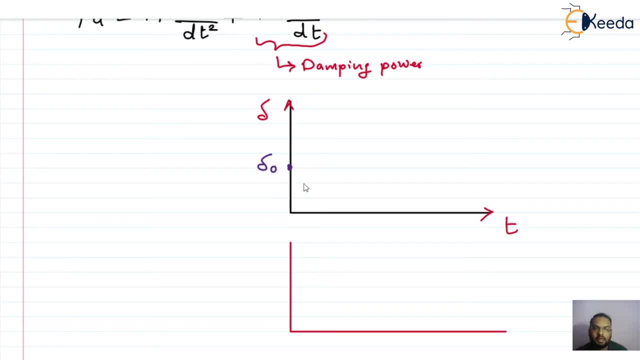 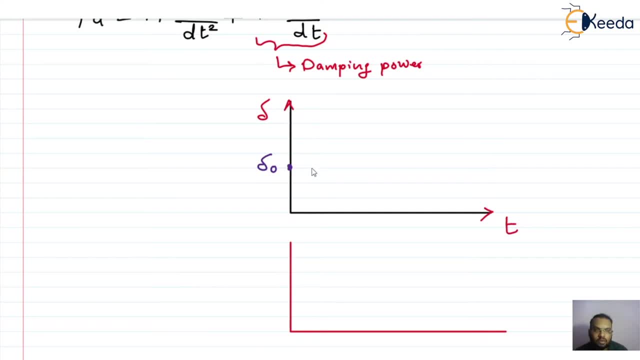 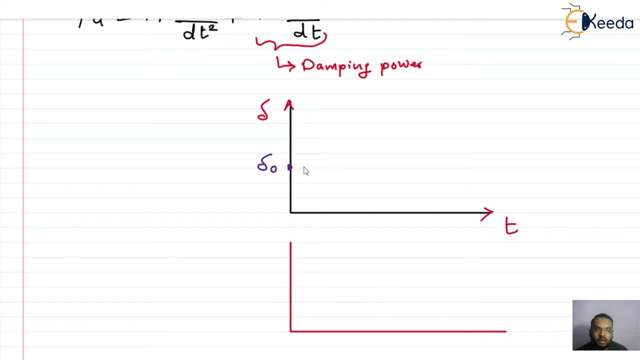 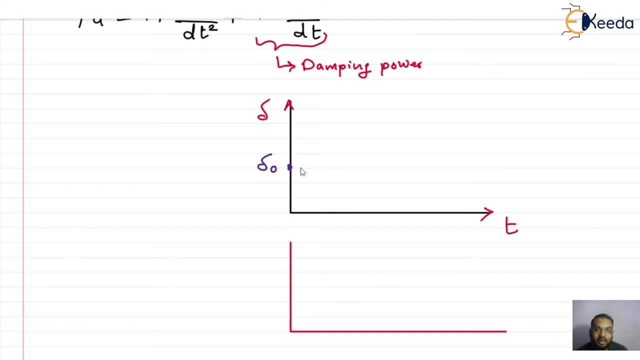 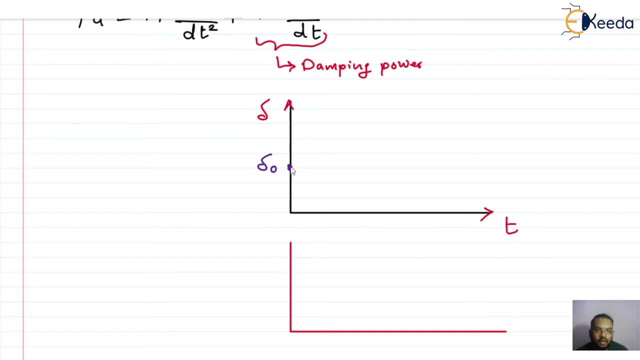 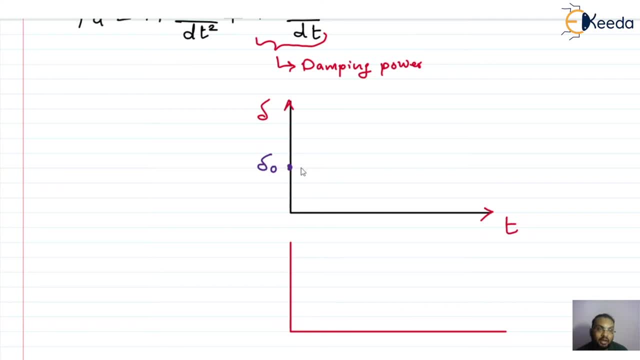 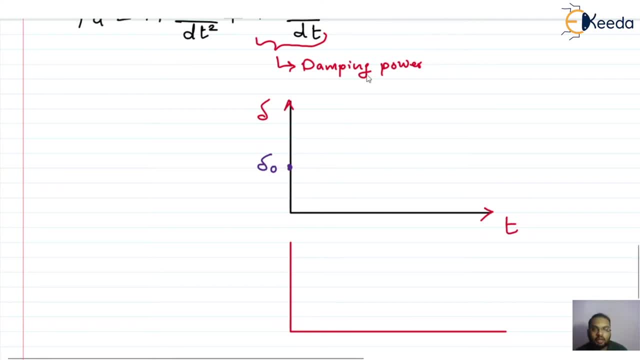 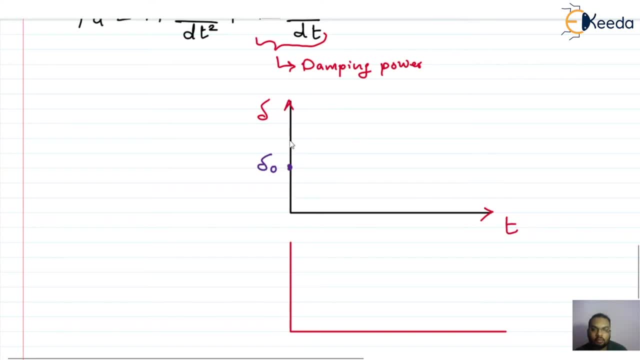 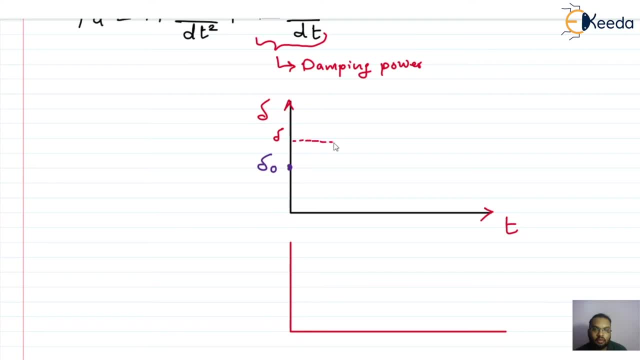 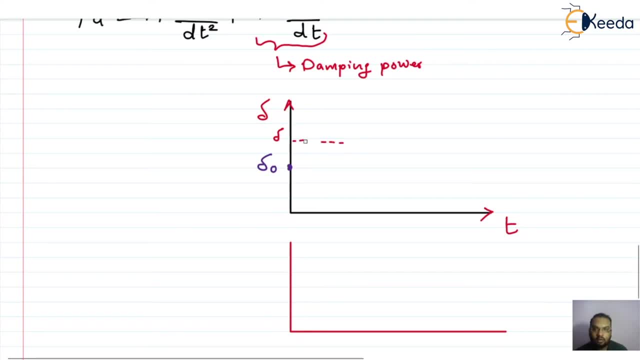 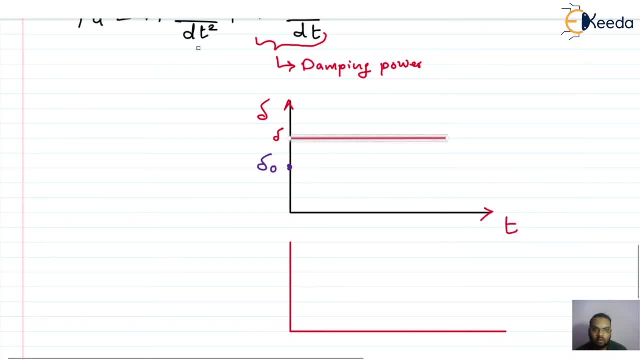 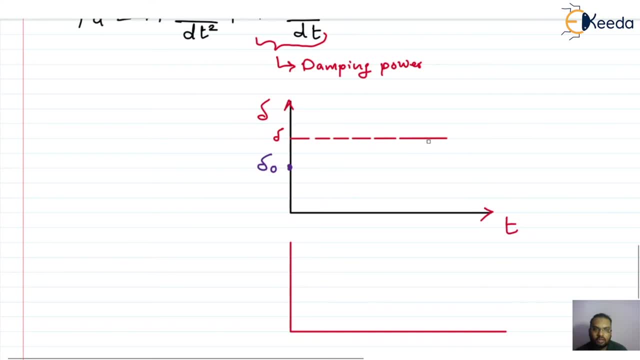 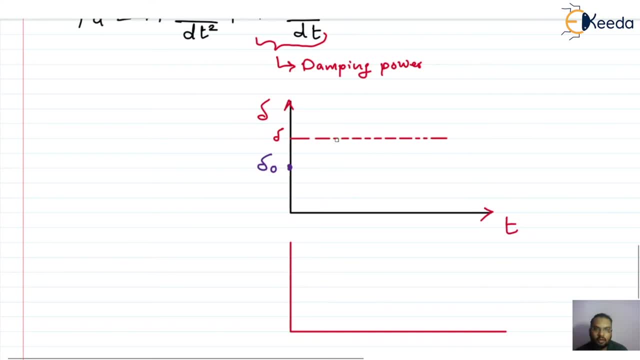 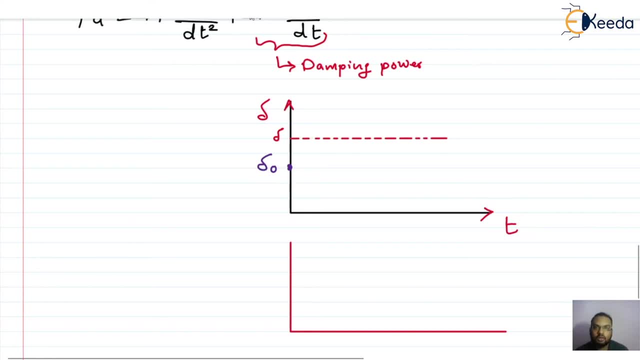 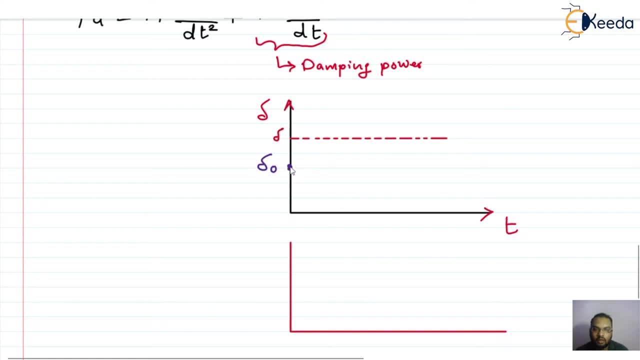 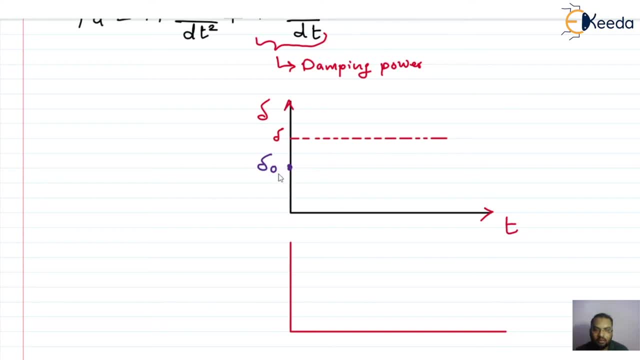 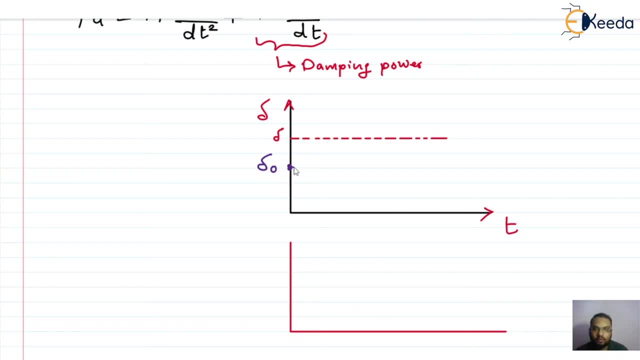 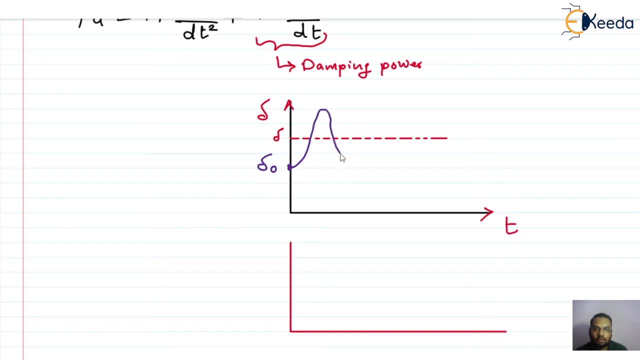 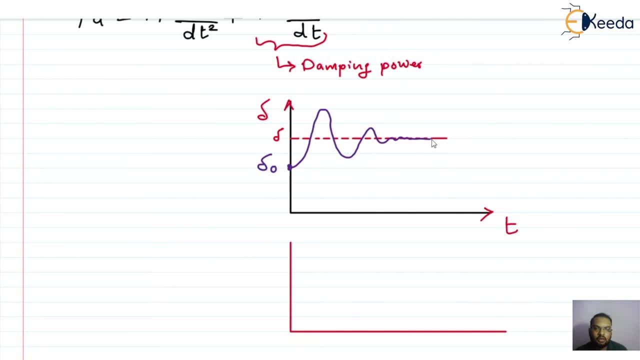 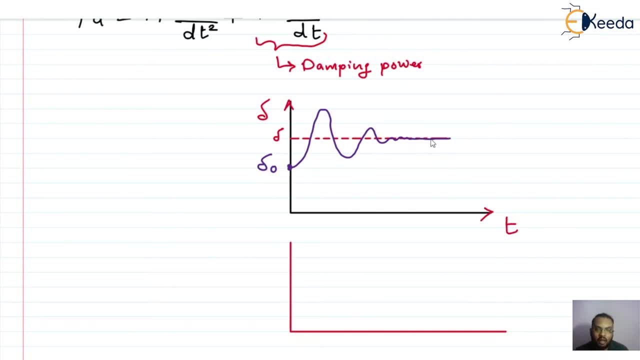 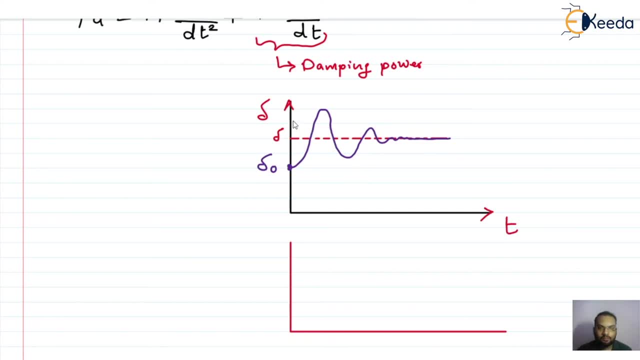 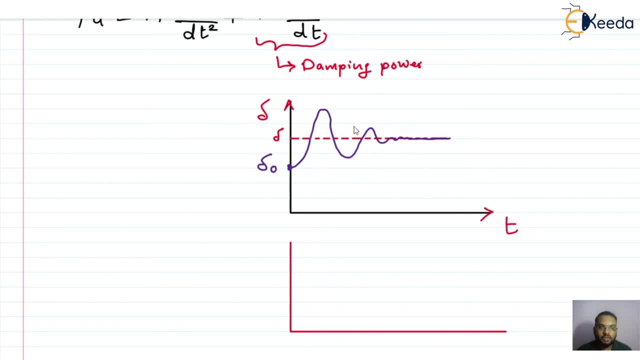 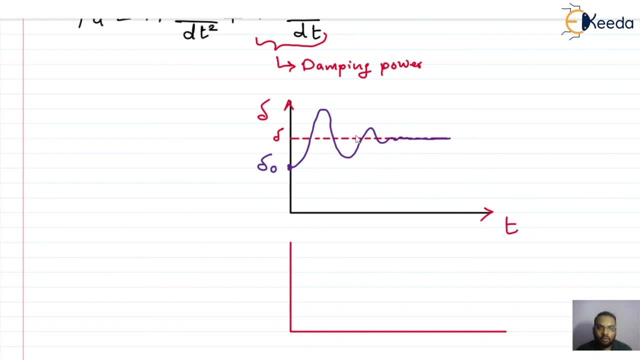 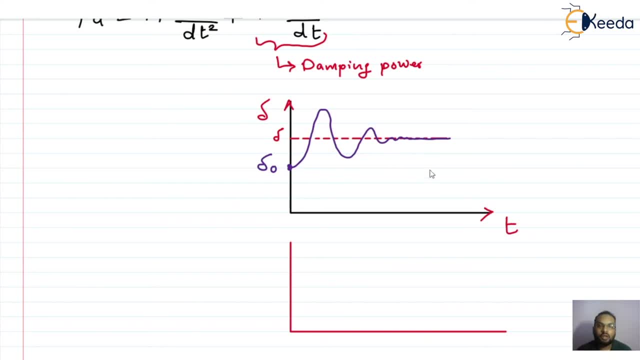 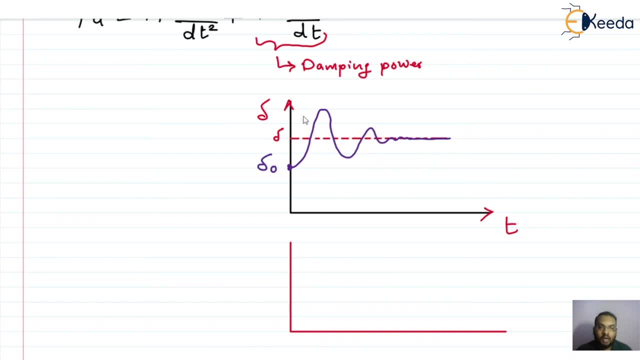 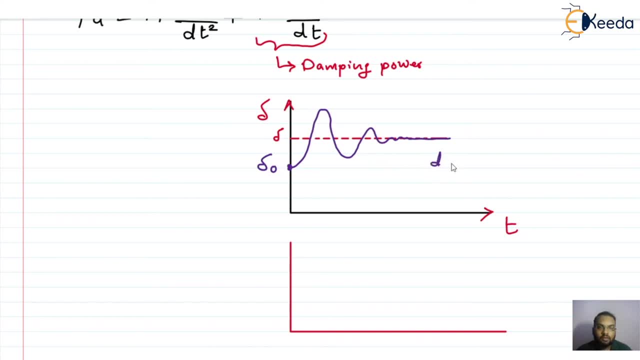 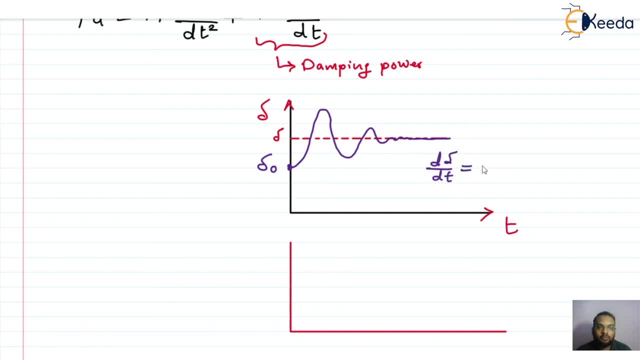 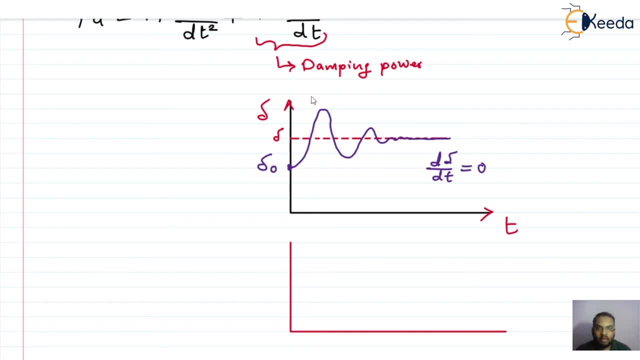 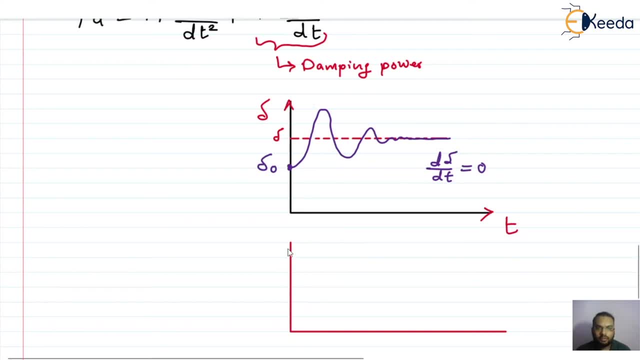 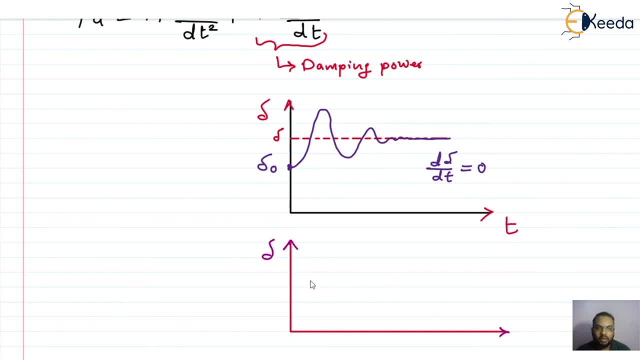 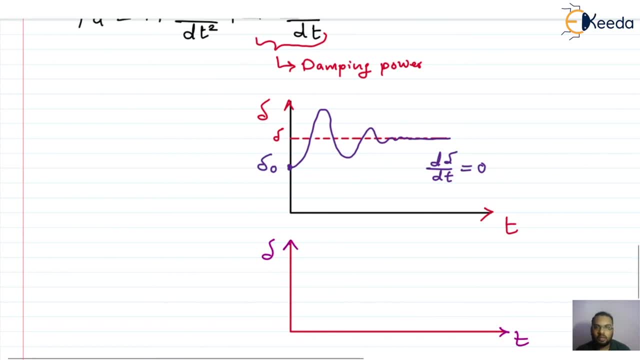 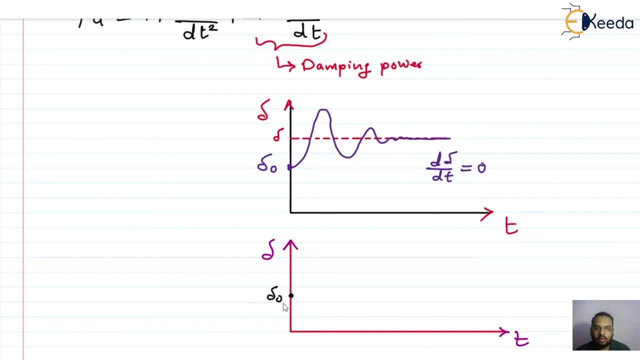 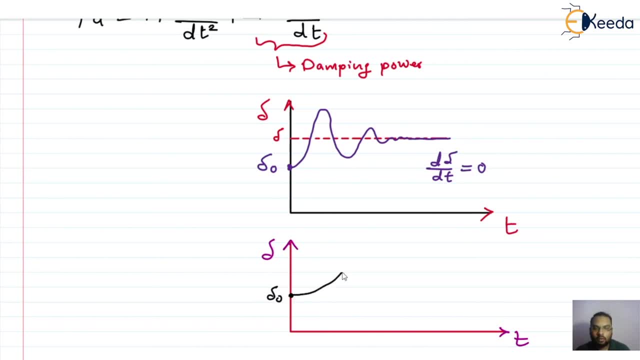 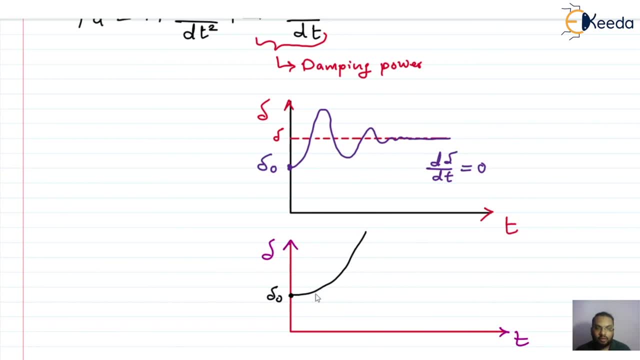 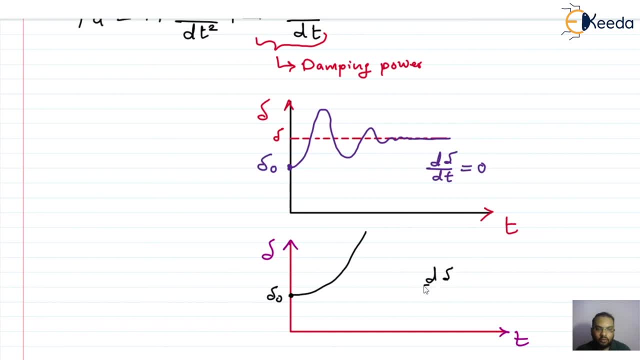 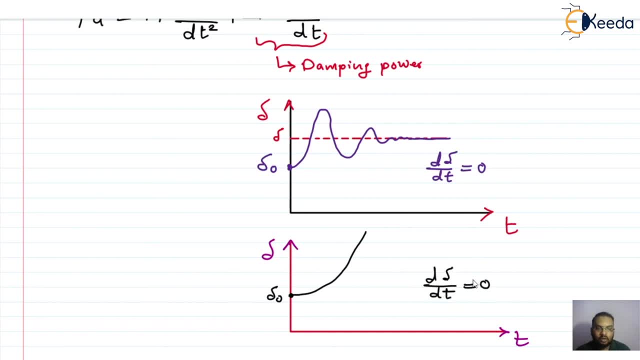